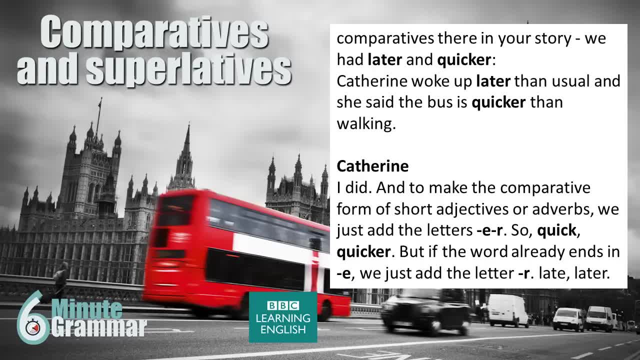 said: the bus is quicker than walking, I did. And to make the comparative form of short adjectives or adverbs we just add the letters er So quick, quicker. But if the word already ends in e, we just add the letter. 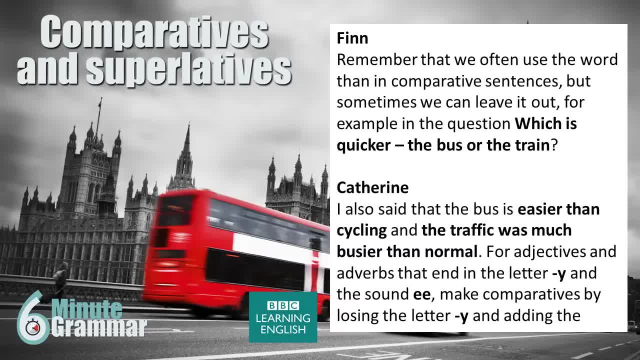 r Late later. Yeah, Remember that we often…. …use the word than in comparative sentences, But sometimes we can leave it out. For example, in the question which is quicker- the bus or the train, I also said that the bus is easier than cycling and the traffic was much busier than normal. 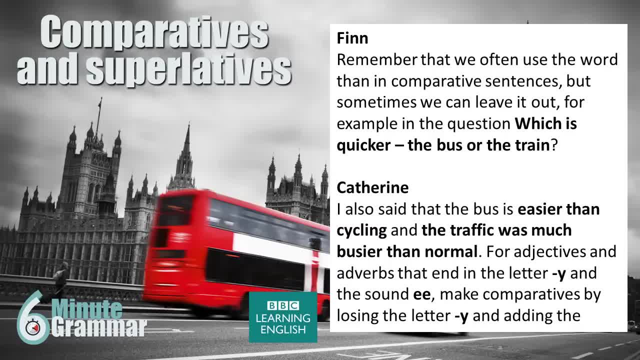 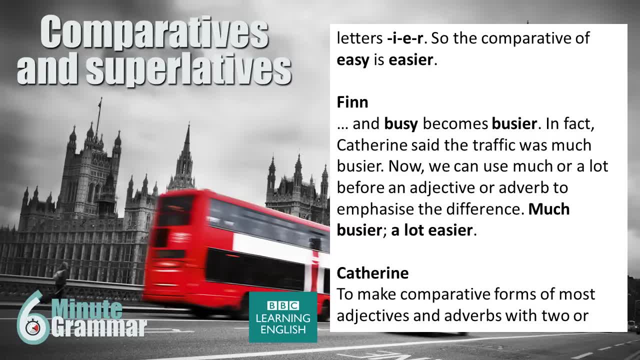 For adjectives and adverbs that end in the letter y and the sound e make comparatives by losing the letter y and adding the letters i, e, r, So the comparatives…. Comparative of easy is easier And busy becomes busier. In fact, Catherine said the traffic was much busier. Now we 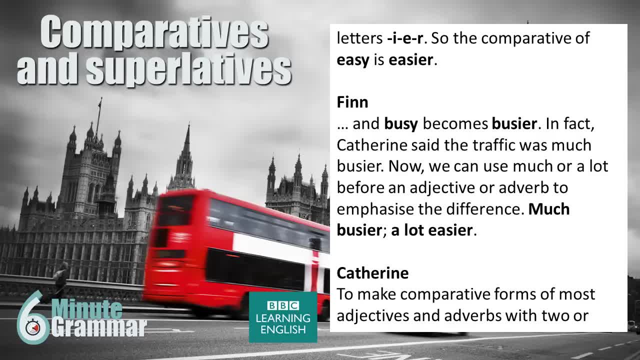 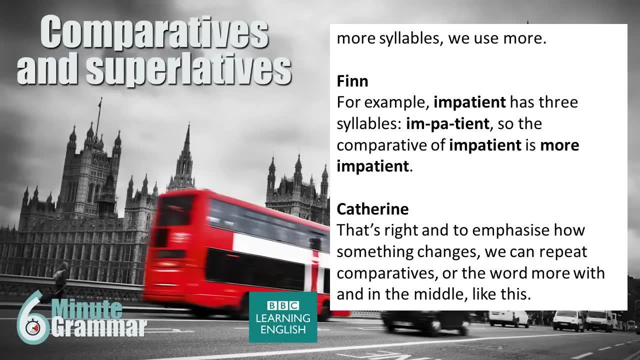 can use much or a lot before an adjective or adverb. to emphasise the difference Much busier, a lot easier To make comparative forms of most adjectives and adverbs with two or more syllables. we use more, For example…. 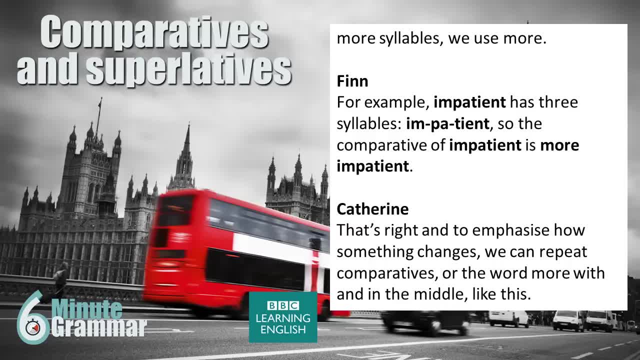 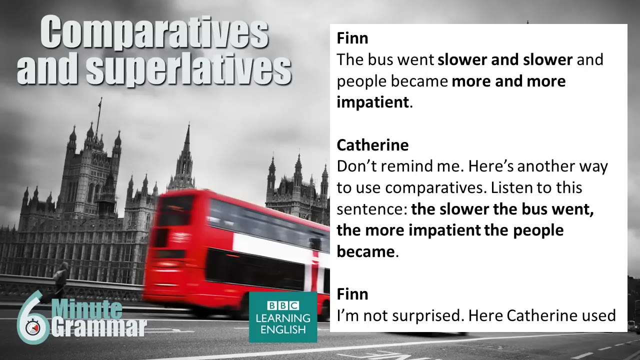 Impatient has three syllables: Impatient, So the comparative of impatient is more impatient. That's right. And to emphasise how something changes, we can repeat comparatives or the word more with and in the middle, like this: The bus went slower and slower and people became more and more impatient. 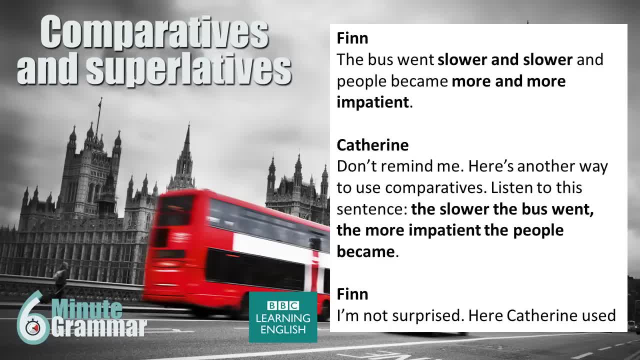 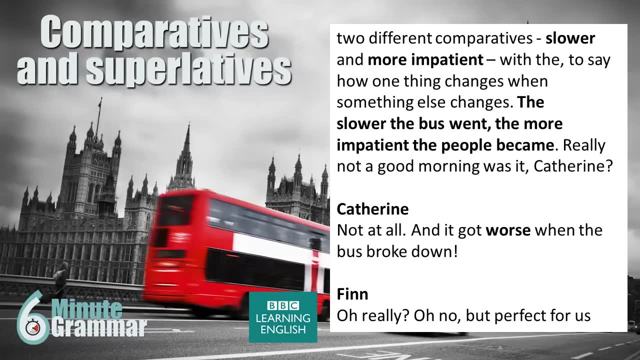 Oh, don't remind me. Here's another way to use comparatives. Listen to this sentence: The slower the bus went, the more impatient the people became. I'm not surprised. Here Catherine used two different comparatives – slower and more impatient with the to say how one thing changes when something else changes. So the slower. 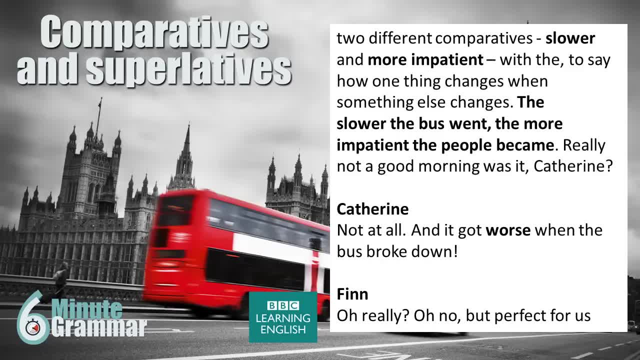 the bus went, the more impatient the— people became. Really not a good morning, was it, Catherine? Not at all, And it got winner, winner and no loser. She's got that right, al Malcolm, husband, I see. So she applied those two jobs to each other, and I wanted to express how she worked hard to get rid of everybody else who has complaints in order to improve the causality of Sh diyorum, How's that for you, Catherine? 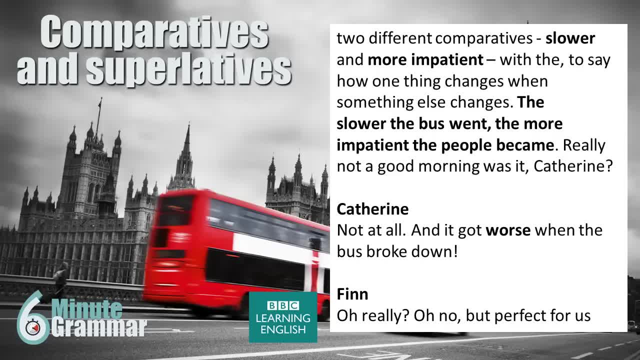 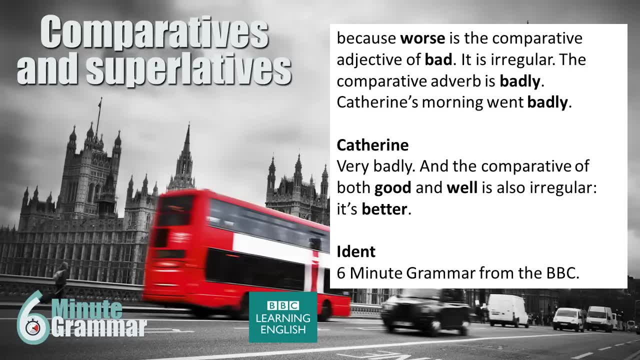 Not at all. And it got worse when the bus broke down. Really, Yes, I couldn't believe it. But perfect for us, because worse is the comparative adjective of bad. It's irregular, The comparative adverb is badly. Catherine's morning went badly. 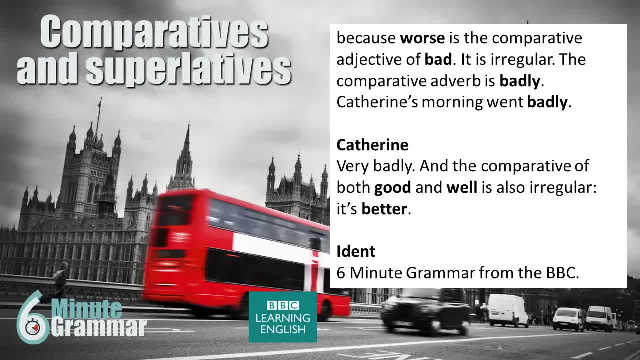 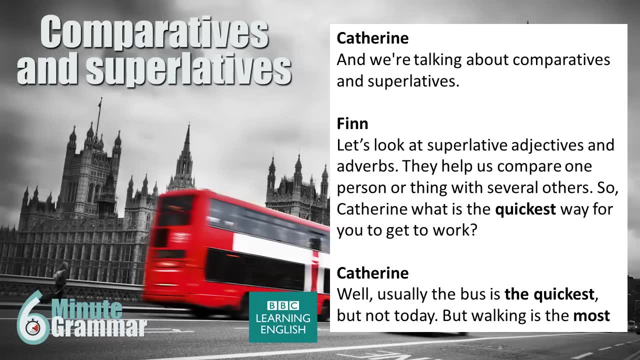 Very badly, And the comparative of both good and well is also irregular. It's better. And we're talking about comparatives and superlatives. Let's look at superlative adjectives and adverbs. They help us compare one person or thing with several others. 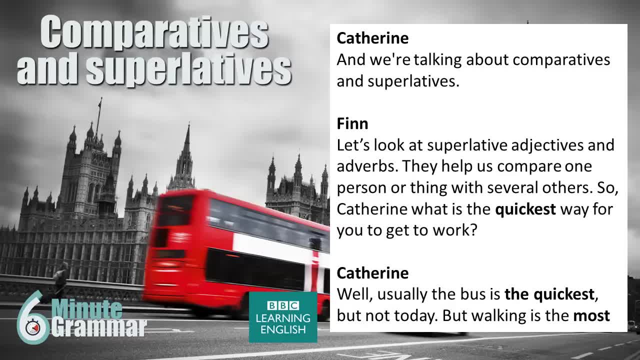 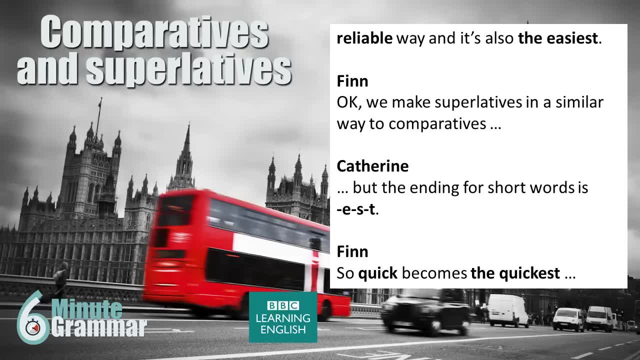 So, Catherine, what is the quickest way for you to get to work? Well, usually the bus is the quickest, but not today. But walking is the most reliable way and it's also the easiest. OK, We make superlatives in a similar way. 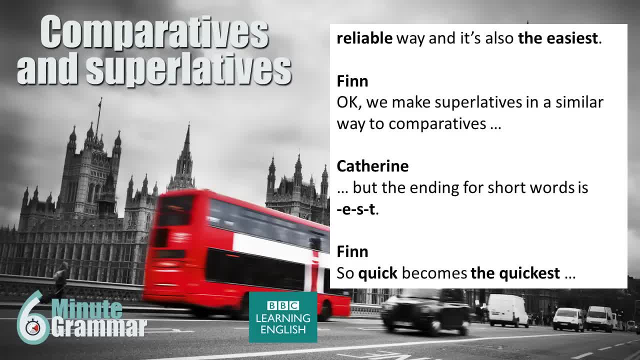 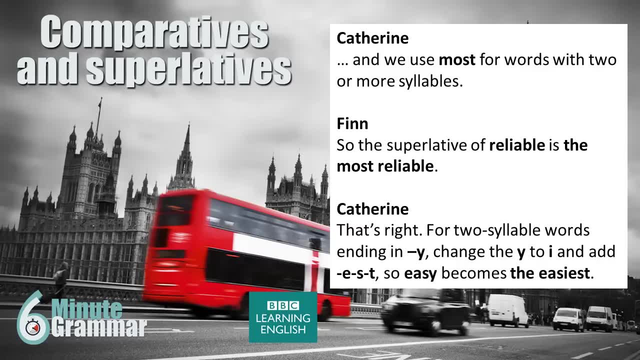 But the ending for short words is est, So quick becomes the quickest, And we use most for words with two or more syllables. So the superlative of reliable is the most reliable. That's right Now for two-syllable words ending in the letter y. 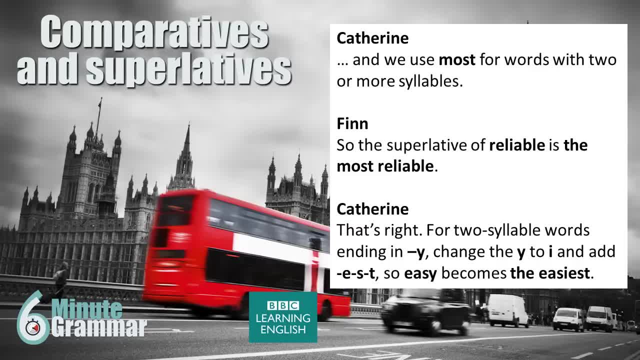 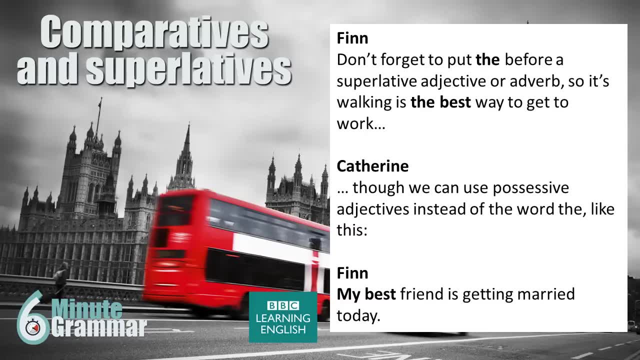 change the y to i and add est, So easy becomes the easiest. And don't forget to put the before the Or a superlative adjective or adverb. So it's walking is the best way to get to work, Though we can use possessive adjectives instead of the word the, like this: 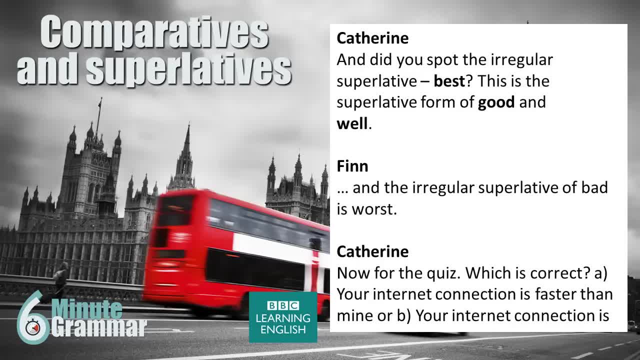 My best friend is getting married today. And did you spot the irregular superlative best? This is the superlative form of good and well, And the irregular superlative of bad is worst. Now for the quiz, Which is correct. 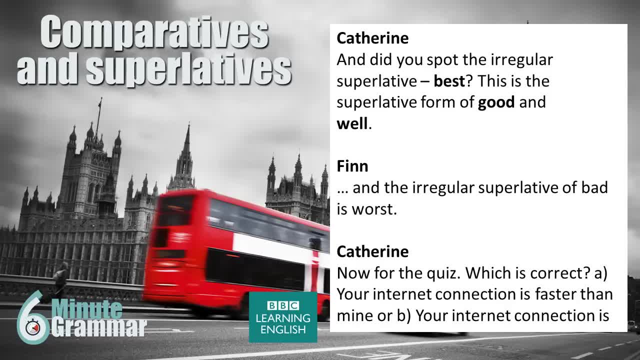 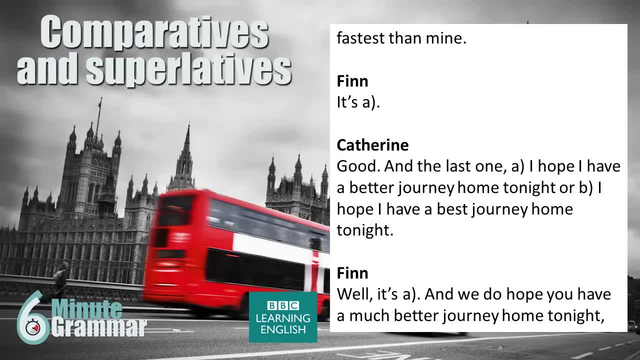 A- Your internet connection is faster than mine, Or B- Your internet connection is fastest than mine. It's A- Good And the last one: A- I hope I have a better journey home tonight, Or B- I hope I have a best journey home tonight.